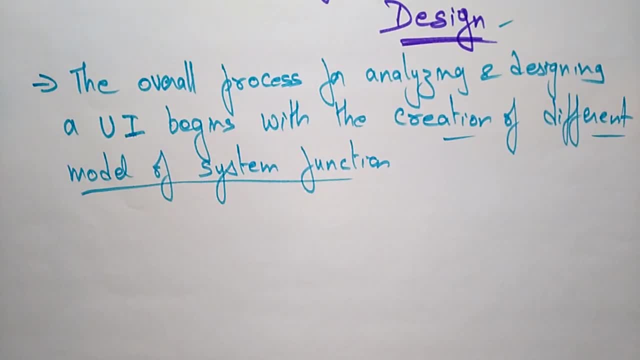 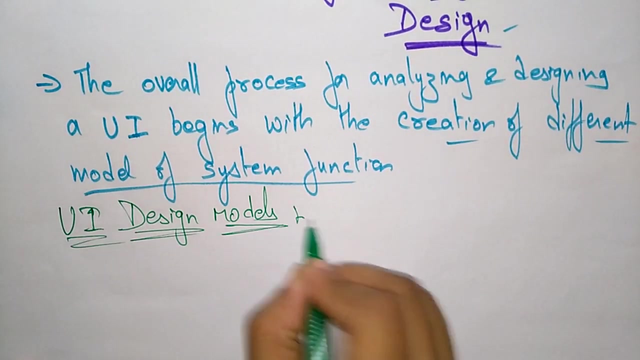 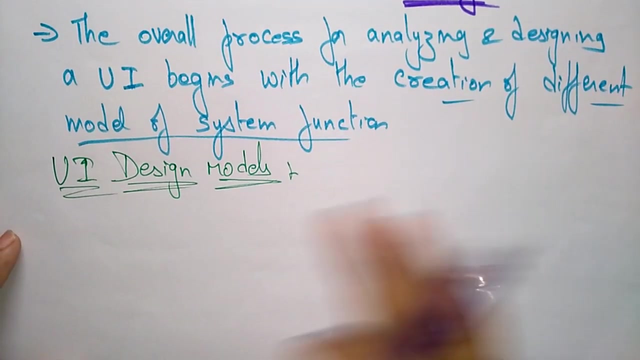 So there are actually the four different models will be present in user interface. Now let us see what are those User interface Design models. So with the help of these design models, we will start the user interface for analyzing and the designing. So there are totally the four different models will be there. 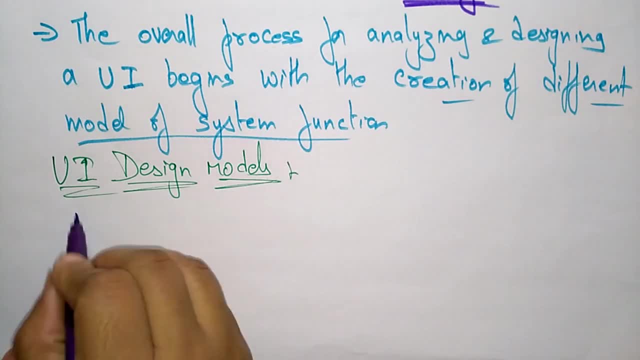 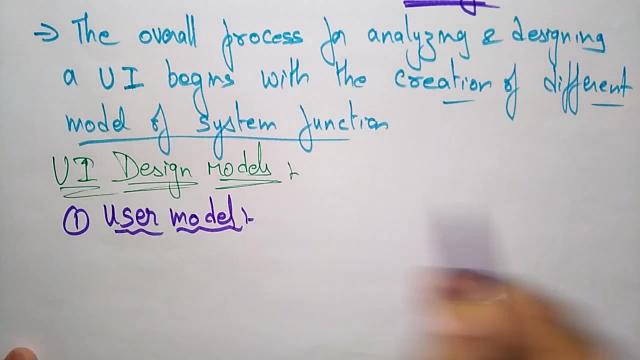 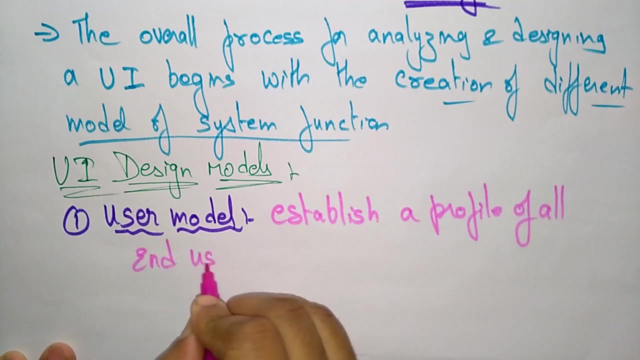 That means the user interface design models will be four. The first one is the user model. The first user interface design model is the user interface User model. So what does this user model will do? This user model will establish a profile of all end users of system. 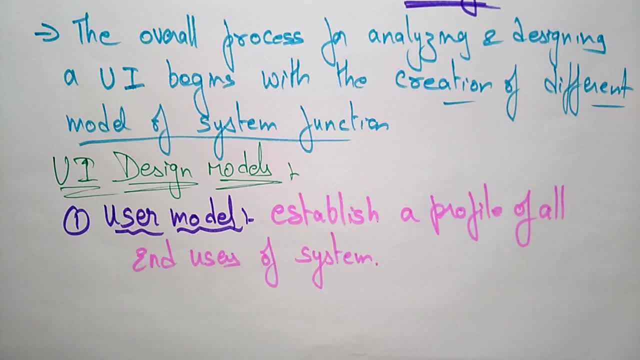 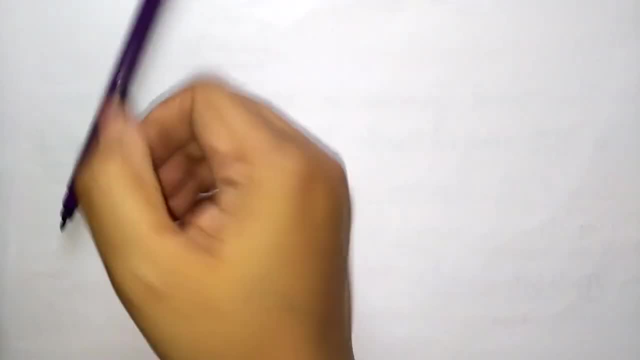 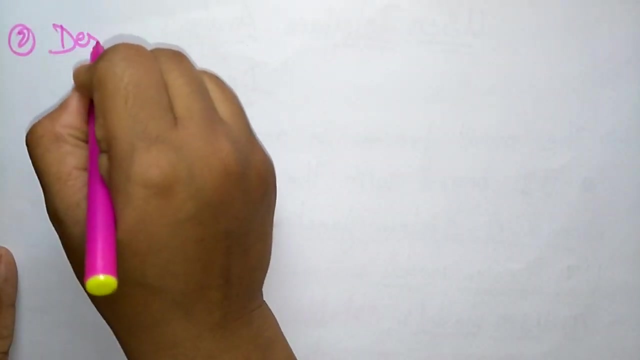 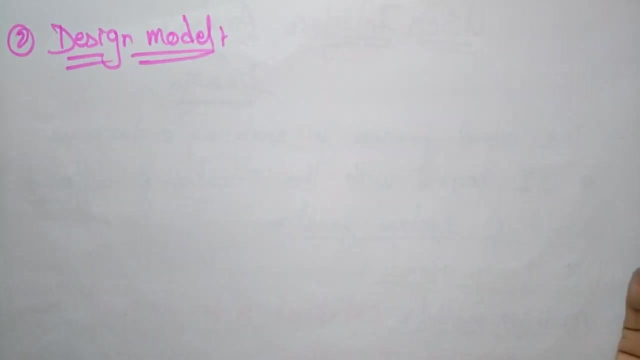 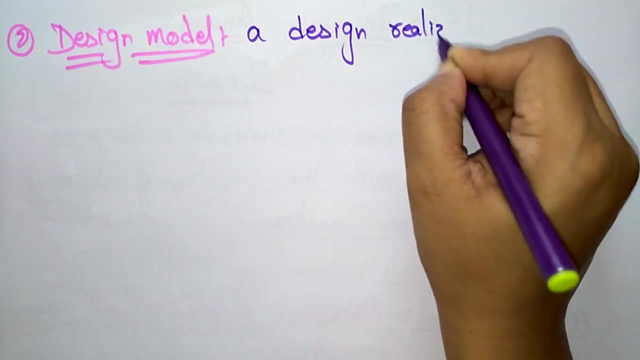 So what this user model will do? This first, the user model will try to establish a profile of all end users of system. So in the second model, The second model was. second is design model. So what this design model will do. A design model- here a design realization of the user model, will be present. 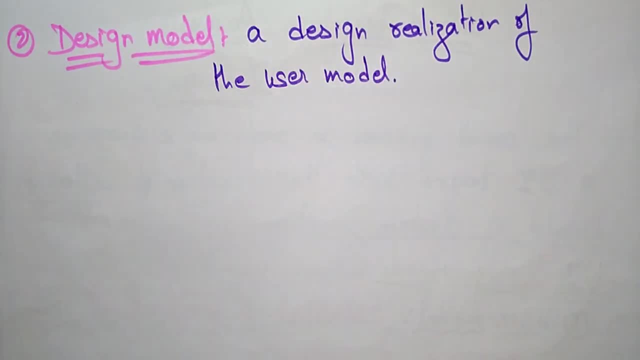 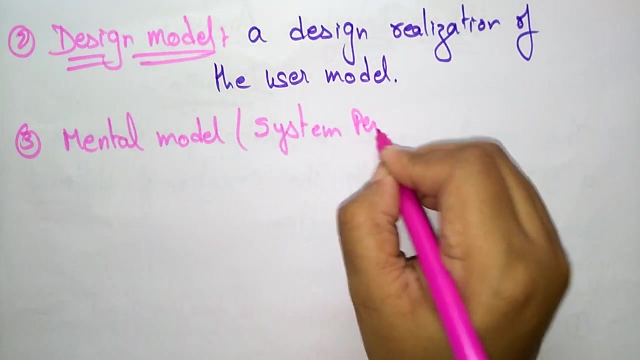 So in the design model, a design realization of user model. whatever the user model will establish, so further, a design realization of user model will be present in the design model. And the third, one third model is mental model. The another name for this mental model is nothing but a system perspective Means in the view of system perception. 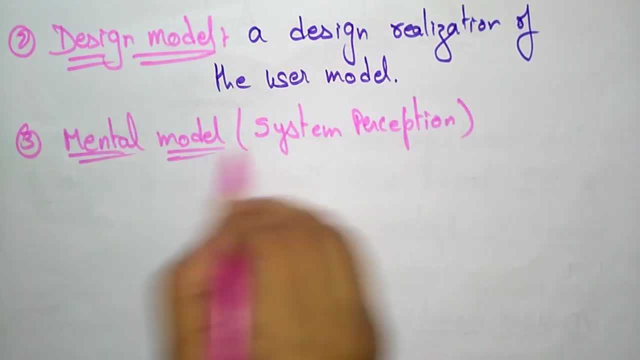 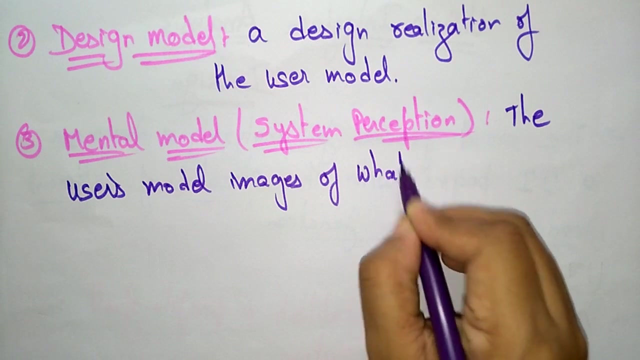 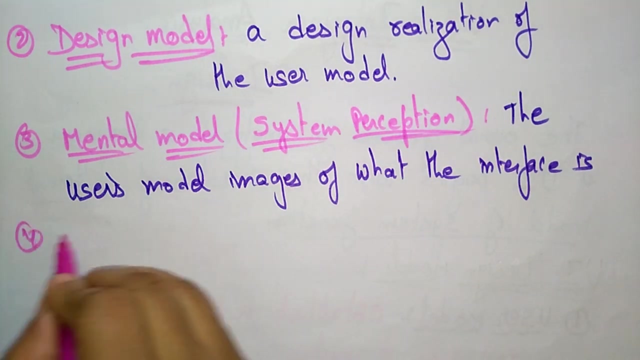 In the view of system perception. So the third model is the mental model. So here the user model. so whatever the user's model, images of what the interface is, Interface is. And the fourth model is the implementation model. Implementation model.